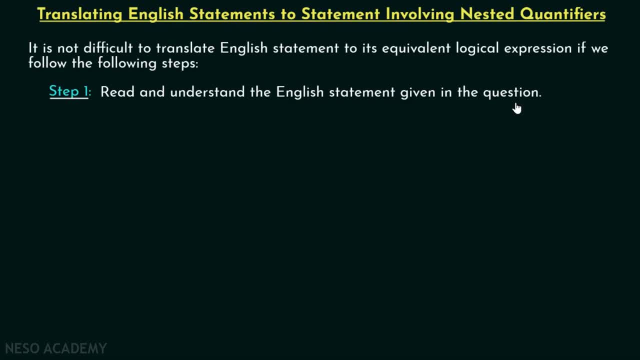 discourse, the quantifiers and the variables in the particular English statement. Okay, now let's see step number two: Find the domain of discourse according to the statement. As you have understood the statement now, it is easier for you to find out the domain of discourse right Now let's see. 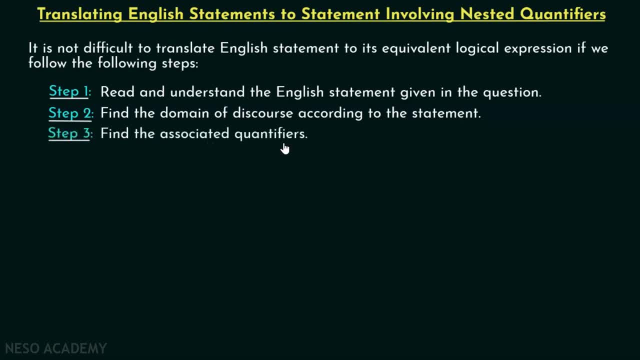 step number three: Find the associated quantifiers. Now it's time to find the associated quantifiers. Right After this, step four is to rewrite the statement so that the domain of discourse and quantifiers are properly visible. This is important step, let me tell you. You have to rewrite the 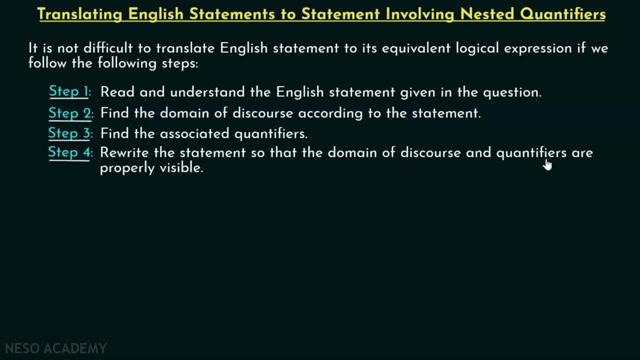 statement so that the domain of discourse and the quantifiers must be visible. After this, the final step is to introduce the variables in the statement, And that's it. After this step five, you could see the statement properly and you would be able to convert it into its equivalent. 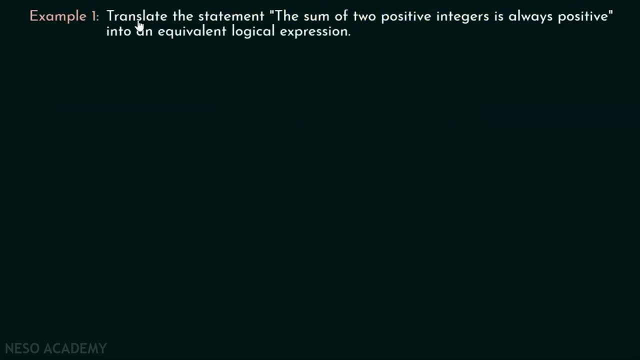 logical expression. Now let's see one example: Translate the statement the sum of two positive integers is always positive into an equivalent logical expression. Now our job is to translate this statement, that is, the sum of two positive integers is always positive, to its equivalent logical expression For this: 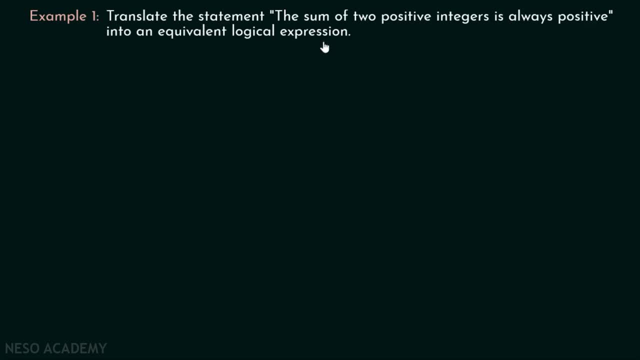 of course, we will follow all the five steps which we have seen already. right, Let's just see the statement. once again, The sum of two positive integers is always positive. Step one is to read and understand the statement. right, We first read the statement and understand the. 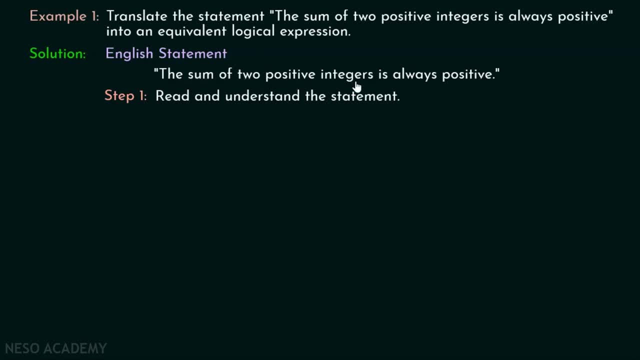 statement. Let's read the statement once again. The sum of two positive integers is always positive. Now let's just try to understand it. Here we are talking about two positive integers. The sum of two positive integers is always positive. no matter what which two integers you will take, Their sum will always be positive. 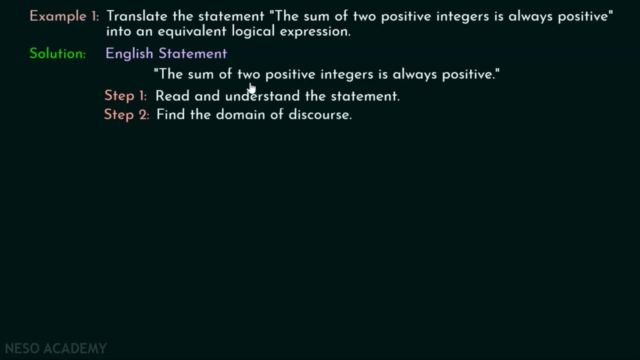 right, Let's see step number two. As you have understood the statement, now it's time to find the domain of discourse. Here you're talking about integers, right, And that two positive integers, or you can take integers also. Now step three is to find the associated quantifiers. You can see that in this statement. 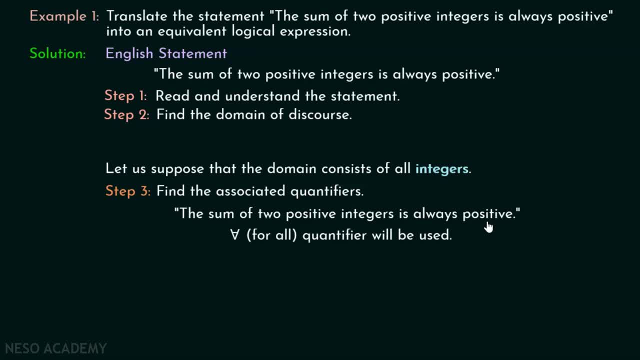 the sum of two positive integers is always positive. We are actually talking about any two positive integers, no matter what right. So actually we are talking about, for all quantifier. This is a general statement. The sum of two positive integers is always positive. 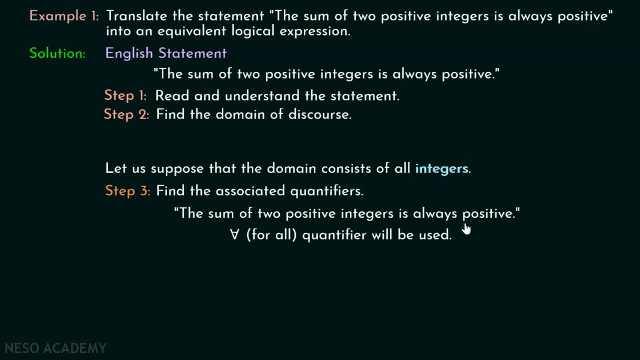 You're not talking about few positive integers. You're not talking about there exists some positive integers. You're talking about all positive integers, no matter what Right. Therefore, we will use for all quantifier. okay, Now, step number four is to rewrite the 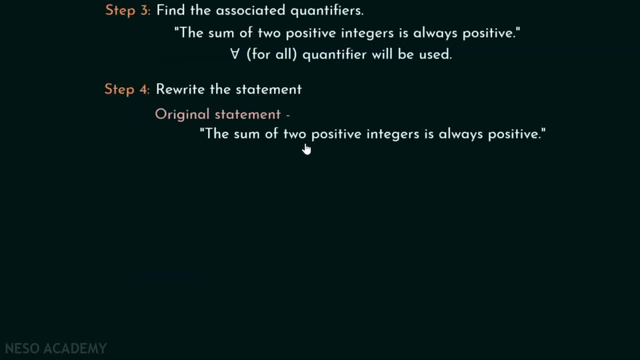 statement. We know that this is the original statement. The sum of two positive integers is always positive. Now we can rewrite this as for every two integers. If the two integers are positive, then their sum is also positive. We know that we want to use for all quantifier. 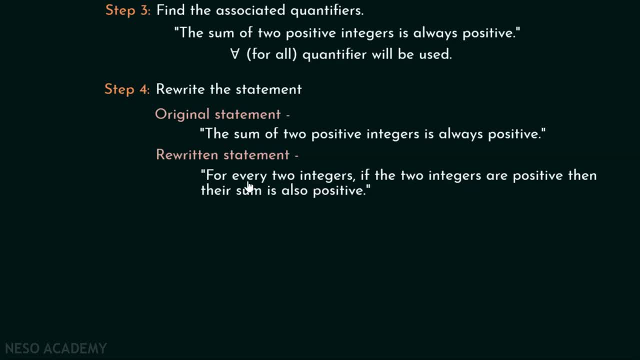 We are talking about every two integers, right. That's why we will write for every two integers. Now, obviously, this is for all. quantifier Implication will come into picture. That's why we will take if-then statement, That is, if the two integers are positive. 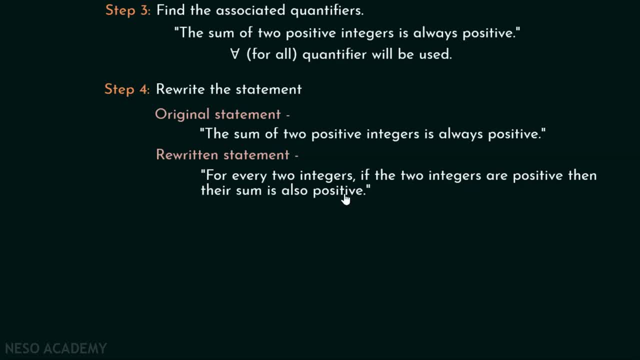 then their sum is also positive, Isn't that? so We are talking about every two integers. First of all, we have to check whether they are positive or not. If the two integers are positive, then their sum will definitely be positive. So the rewritten statement is for every two integers. 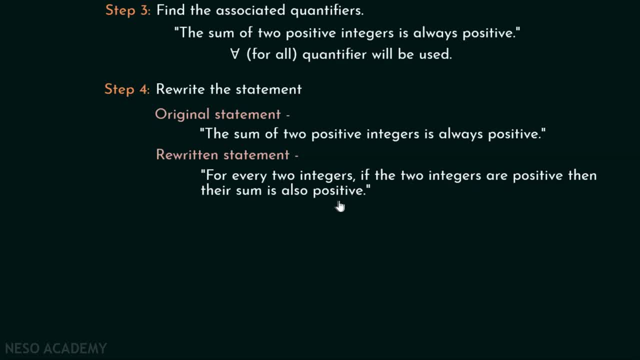 if the two integers are positive, then their sum is also positive. Now let's see step number five, which is introduce the variables. This is the last step. Now, here we are talking about two positive integers, Isn't that so? So we will take two variables. 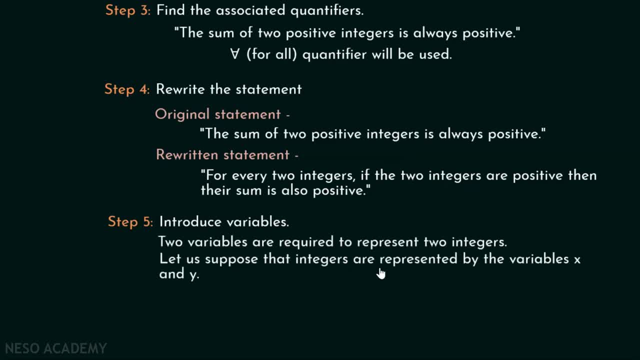 Two variables are required to represent two integers. Let us suppose that the integers are represented by the variables x and y. Then we can rewrite the statement as for every two integers, x and y. if x and y are positive, then x plus y is also positive. right, Now, it is easy. Now you can easily. 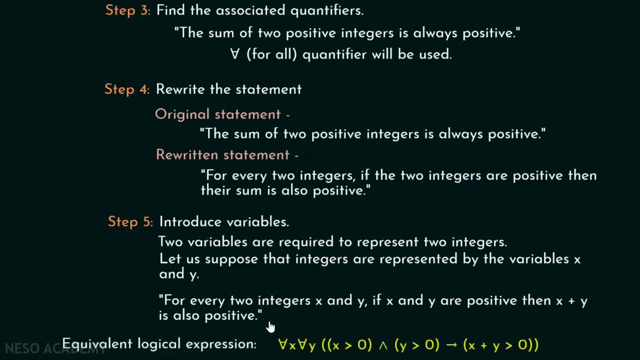 write an equivalent logical expression For all x for all y. That means for every two integers x and y. that means for all x for all y. If x and y are positive, that means if x is greater than zero and y is greater than zero. 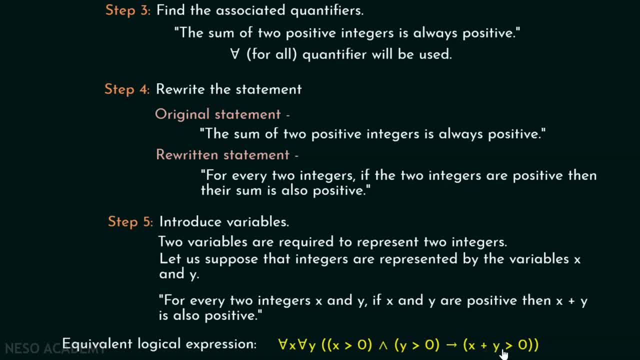 then x plus y is also positive. This means x plus y must be greater than zero. For all x for all y, x is greater than zero and y greater than zero means x plus y is greater than zero. So this is the equivalent logical expression for the statement: the sum of two positive 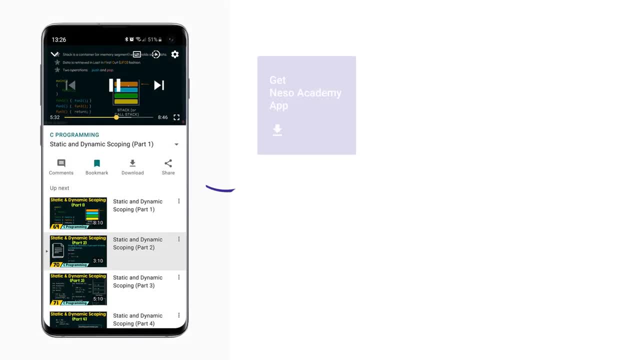 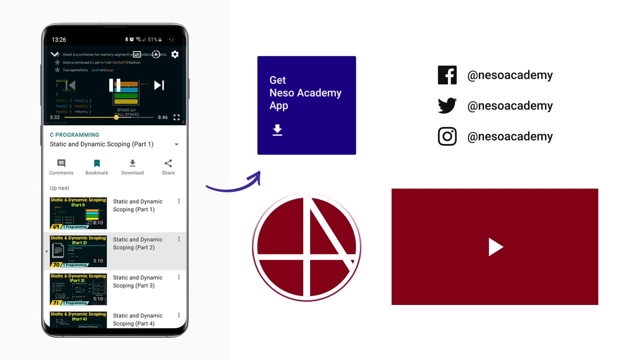 integers is always positive. Thank you for watching.